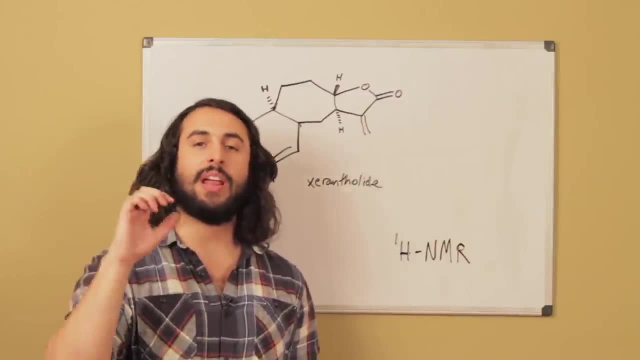 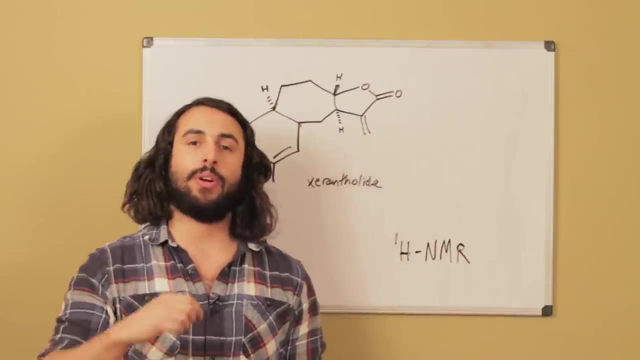 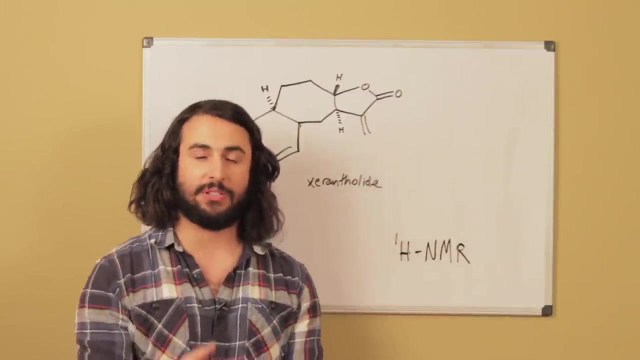 and we can take advantage of that nucleus spin by irradiating or by subjecting a molecule to an external magnetic field, and when we do that we're going to be able to get some very interesting data when we then get spectroscopic data from it. so that is, we induce a magnetic field and then we irradiate with light. 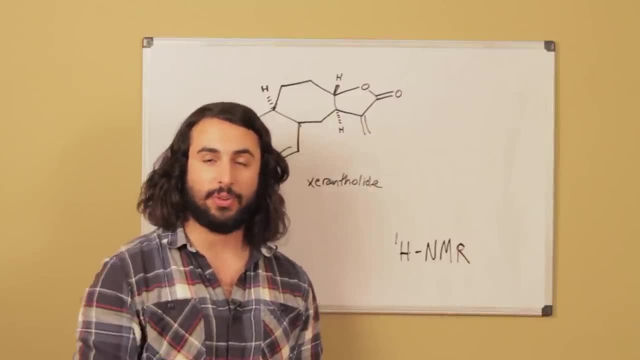 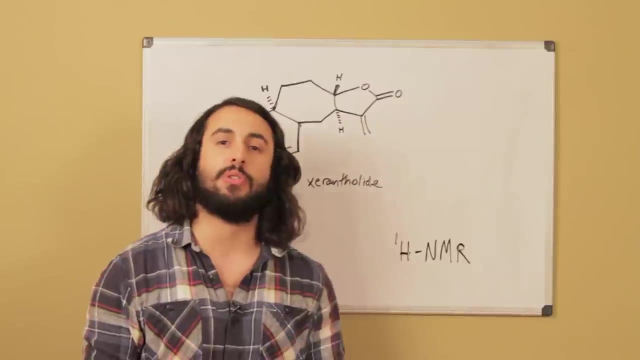 and we gather information about how the light interacts with that compound. so, without getting too into the physics of it all, we're just understanding that we're looking at proton NMR involving protium. these are protium nuclei, so protium, which is a hydrogen isotope of mass one. 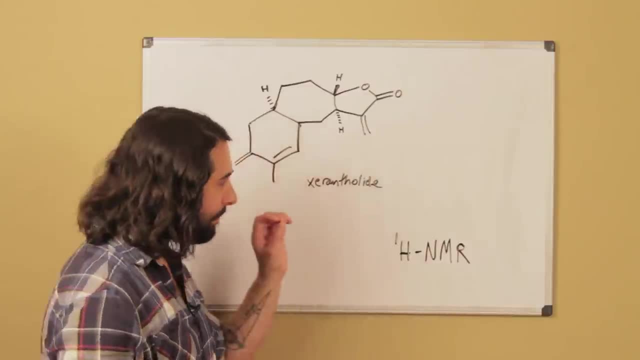 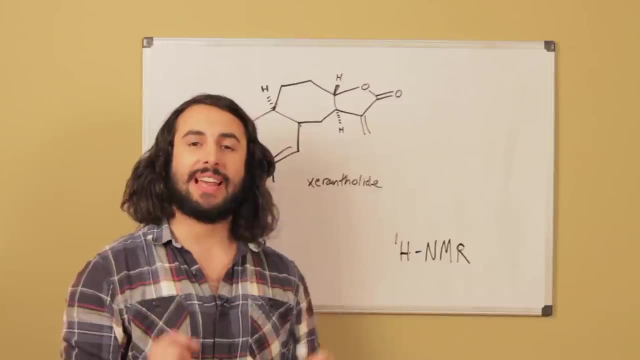 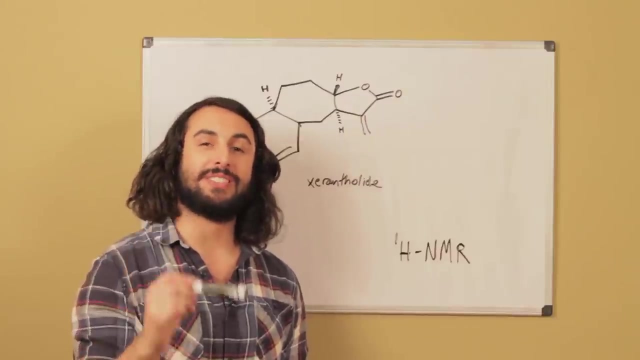 as opposed to deuterium or tritium, and what happens is we're going to be able to irradiate this with light and then get back information that tells us the precise chemical environment of every single proton in this molecule, and we can use that information to discern the precise structure of the molecule. 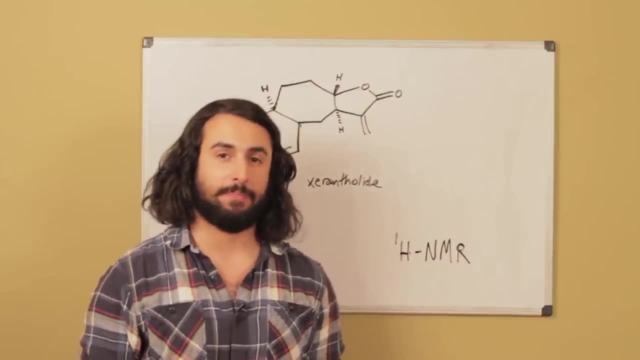 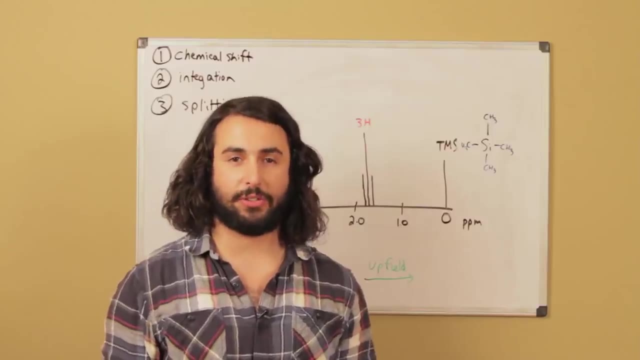 so let's take a look at one of these spectra and talk about how we can interpret them. so what I've done here is I've drawn a sample NMR spectrum and we're going to talk about the three main pieces of data that we are going to try to glean from any NMR spectrum. 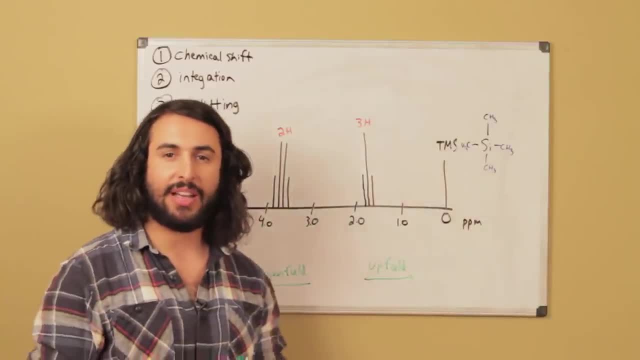 so once again, we're doing this. this is going to be a very simple example. we're not going to get too too in depth, but just in a very basic way, what can we get from an NMR spectrum? so, first of all, what is going on here? 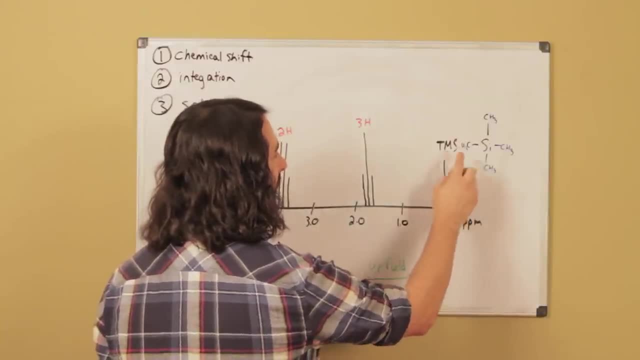 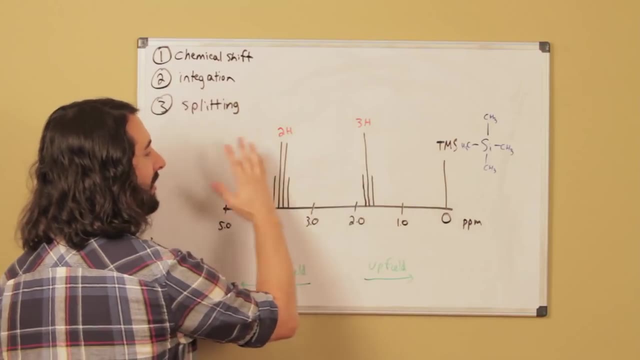 so right here we have a reference peak. this is called TMS, that's tetramethylsilane, and then everything else is given in parts per million, in terms of where it's going to go and where it stands in reference to the TMS. so this is our reference peak. so that's not data. 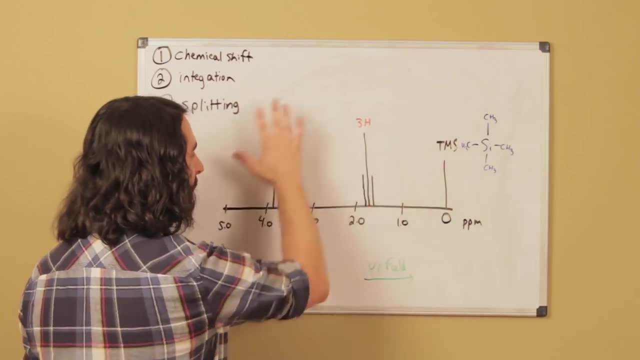 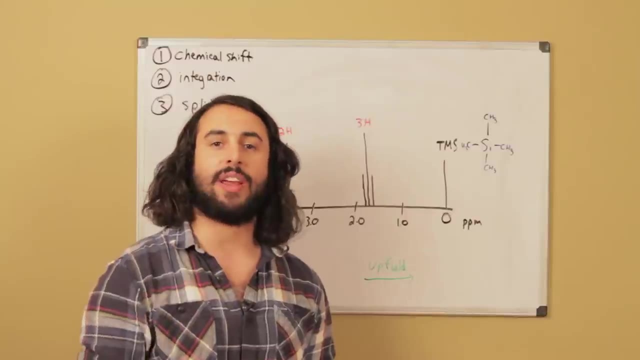 that's going to be on any spectrum. and then this stuff: this is the data. ok, so how is this data? how are we interpreting these peaks, these resonances? well, there's three things that we want to take into account for any resonance on a spectrum. 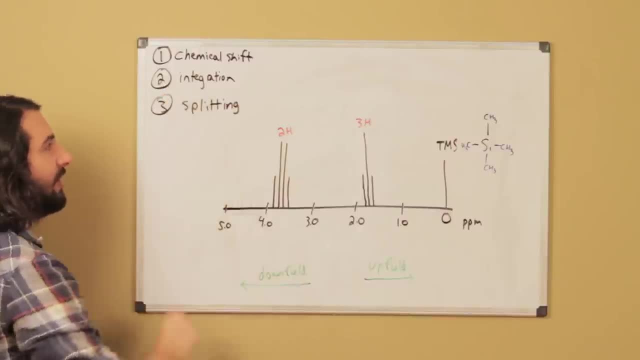 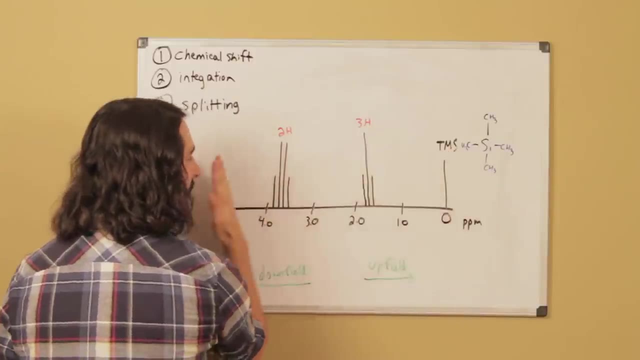 that is going to be the chemical shift, the integration and the splitting. so what do these three things mean? let's talk about them one at a time. so chemical shift. all chemical shift means is: where is it? where is it on the spectrum? is it more downfield or is it more upfield? 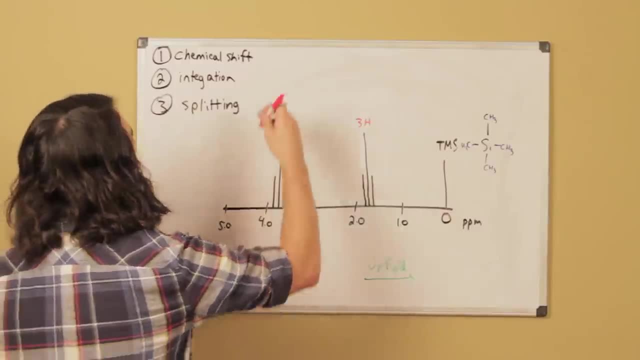 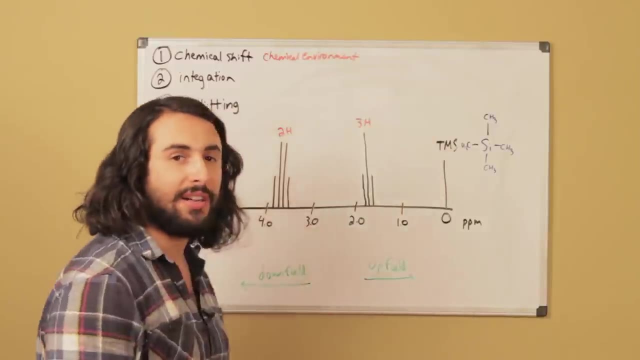 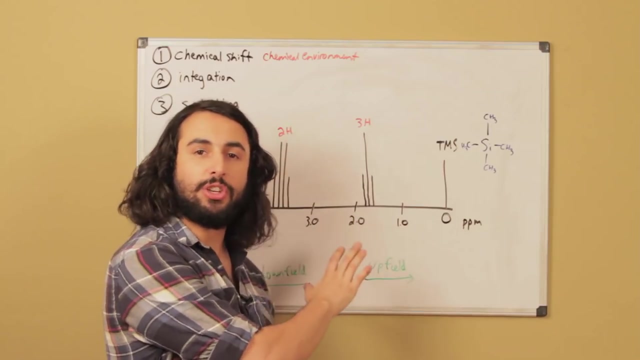 now, what this has to do with is? it tells us about the chemical environment of a particular proton. remember that these are protons that are generating these resonances. so in a molecule, anywhere where there is a hydrogen atom, you are getting some information about the chemical environment of that hydrogen atom. 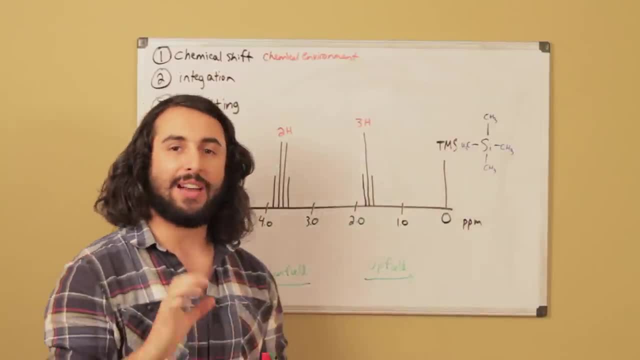 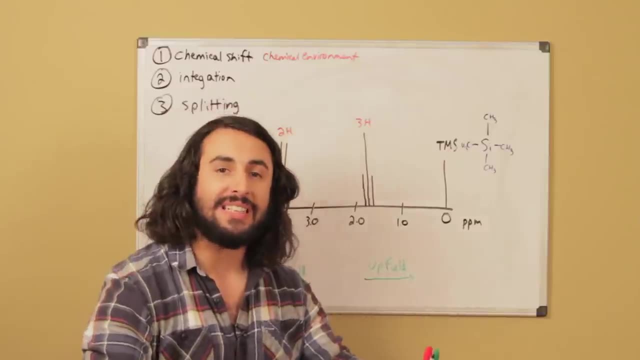 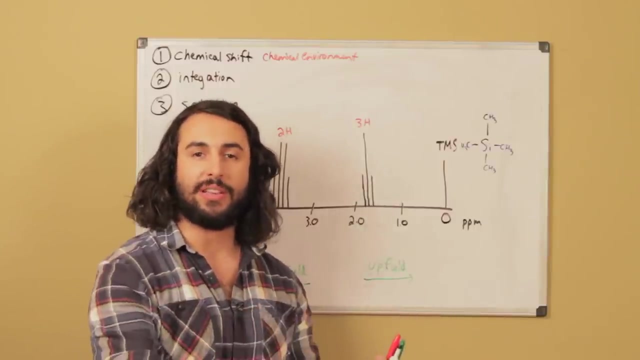 or that proton. so what happens is, the closer that that proton is to some electronegative element, the electronegative atom is going to have a deshielding effect. so because of its electronegativity it is going to withdraw the electron density of that proton away from the nucleus. 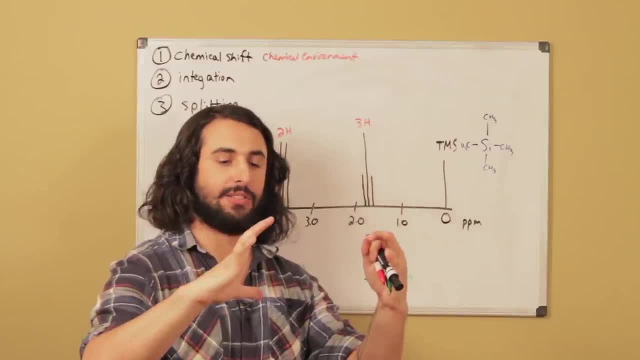 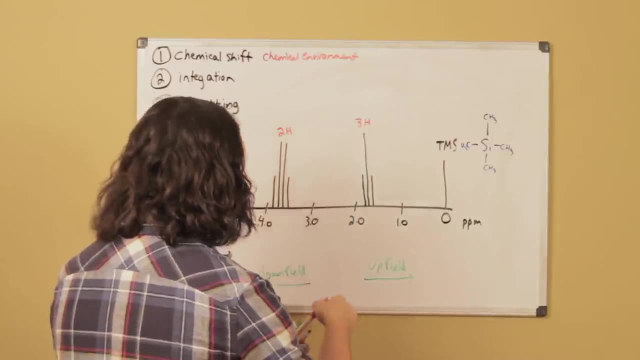 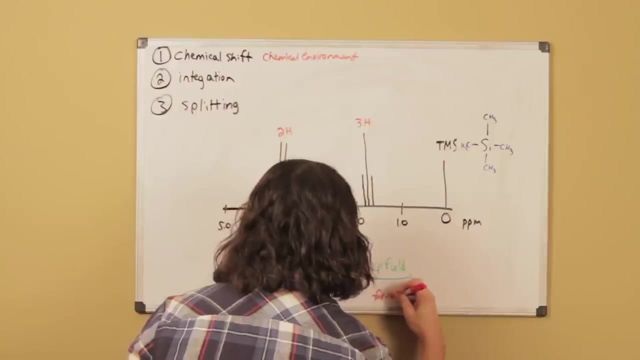 which we call a deshielding effect, because the electrons are moving away from the nucleus and then that will cause that signal to be more downfield. so more downfield means closer to electronegative atoms, upfield means farther away from electronegative elements. 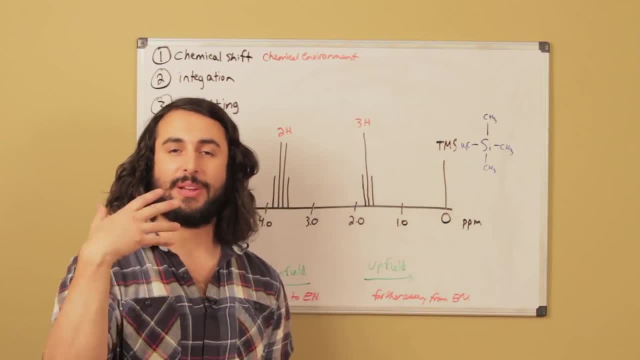 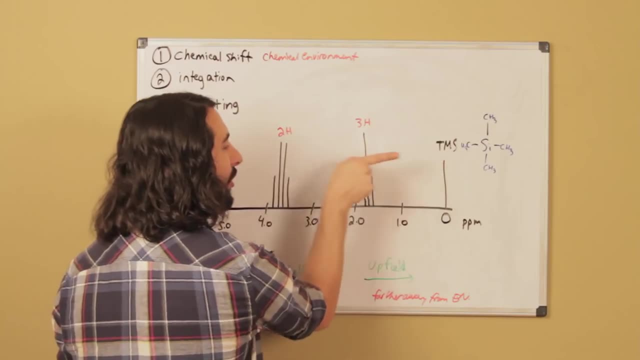 so number one, the chemical shift is telling us about the chemical environment. that means: where is it on the spectrum? this way is closer to electronegative elements. this is further away from electronegative elements. number two is integration. so let's say that we have some chemically equivalent protons. 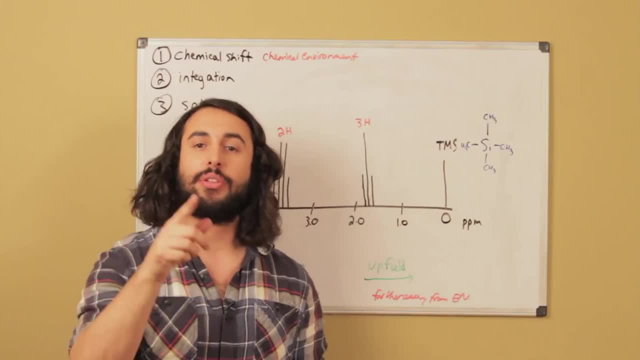 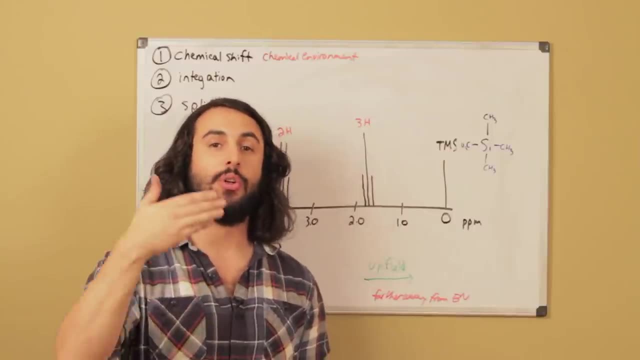 that might be three protons on the same methyl group. as they're spinning around, they see the same thing. as they look down the rest of the molecule, they are experiencing an identical chemical environment. so what ends up happening is, let's say we have one proton on that methyl group. 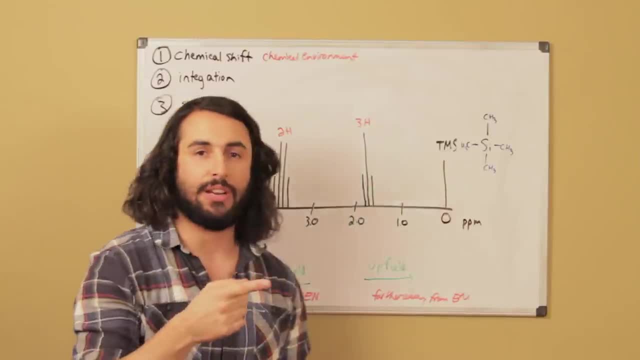 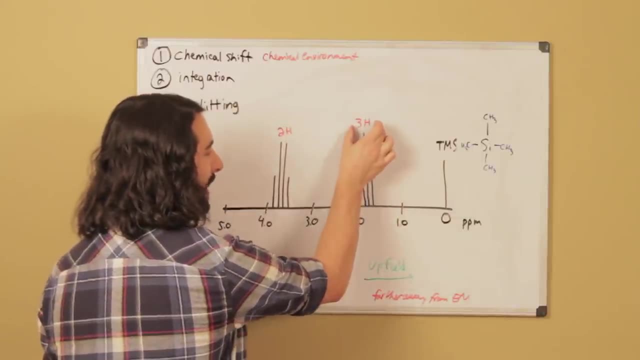 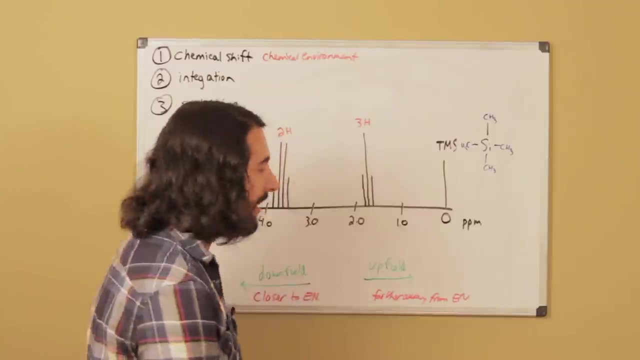 that generates this resonance, generates this information right here. then that second proton also generates the same resonance, so that just enhances this peak and it will get bigger. and then that third proton also generates the exact same resonance or the exact same data, so that too will cause this to grow. 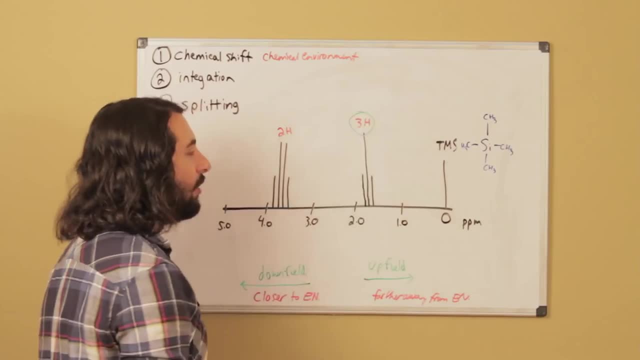 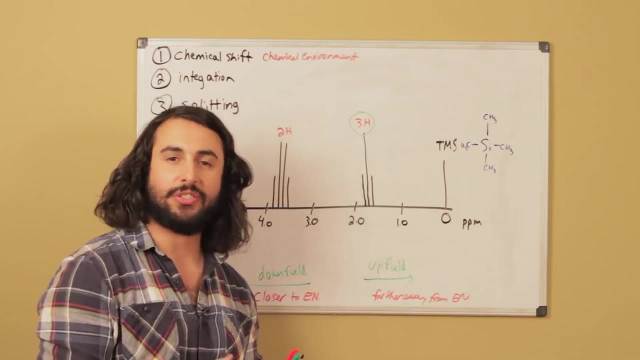 and what that means is: this is an integration. so integration literally means the area under the curve. so NMR spectra don't look exactly like this. this is an oversimplified view of it, but whatever data is happening under that peak, the integration means the area under the curve. 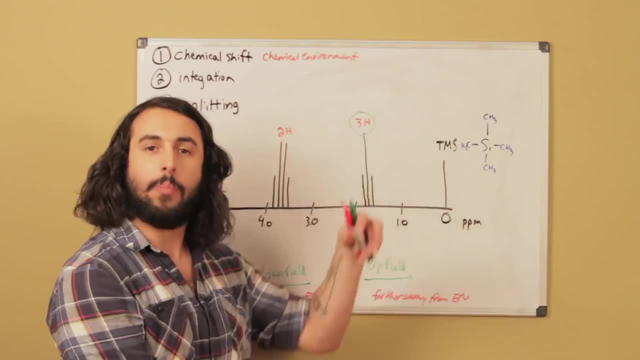 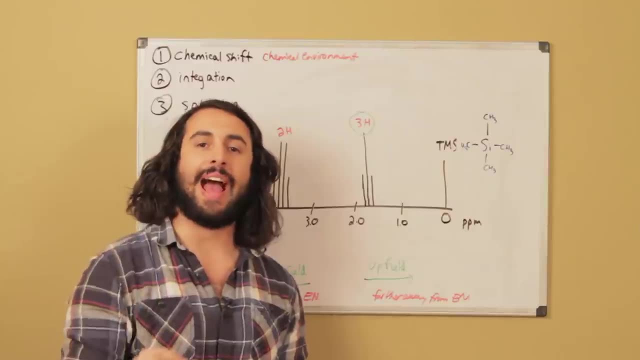 so we can just consider it to be kind of how tall is it or how big is the resonance? and so that's the second bit of information- is the integration. the integration is telling us how many chemically equivalent protons are generating that peak. so if this is integrated to two, 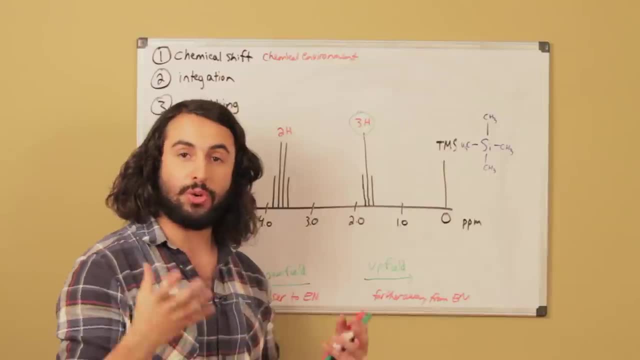 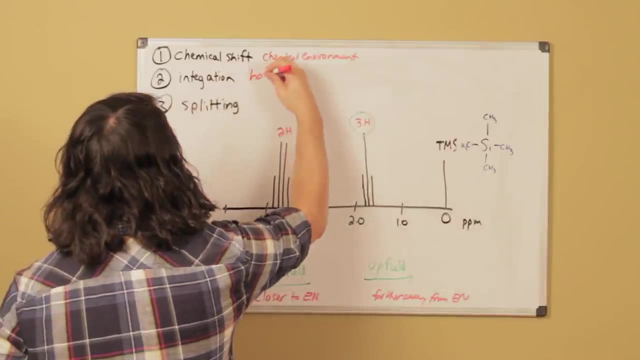 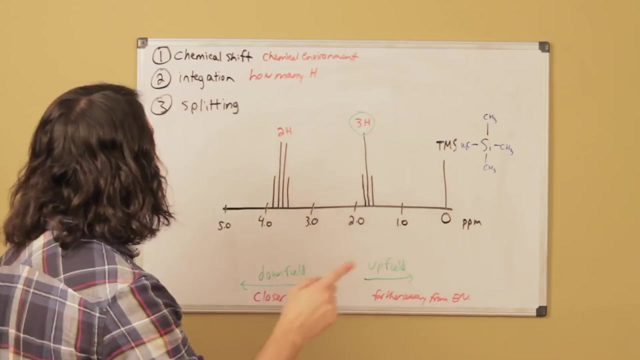 and this is integrated to three, then what we are saying is that two chemically equivalent protons are making that one and three are making that one. so that's integration. that's saying how many protons are generating that peak. now the last thing we want to talk about is splitting. 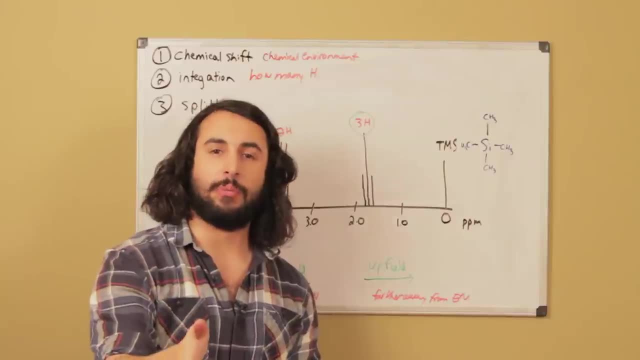 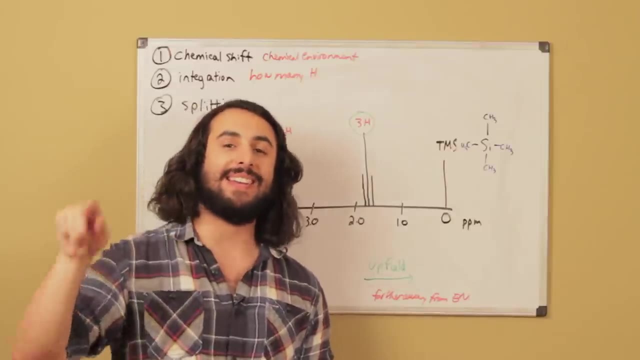 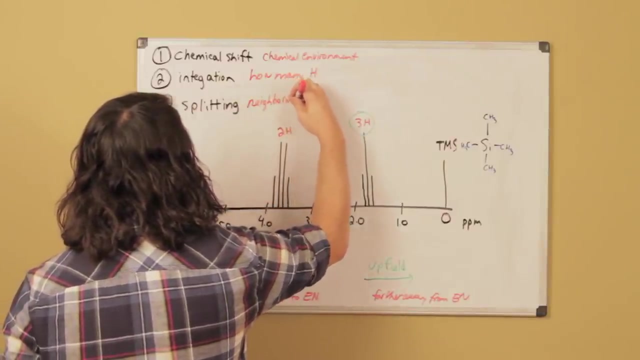 and so chemically equivalent protons will generate the same resonance, but then that resonance will be split into a certain number of smaller peaks, depending on neighboring protons, and so what we want to understand is: so this is about neighboring protons, and this is the N plus one rule. 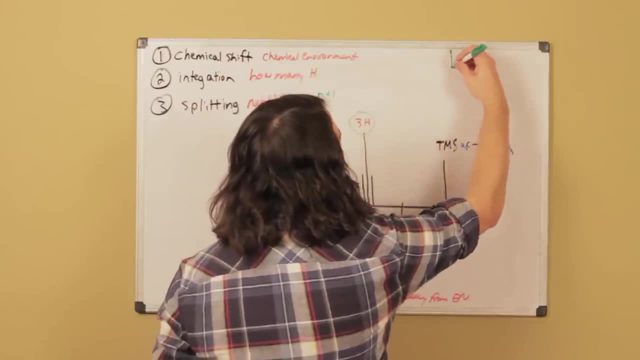 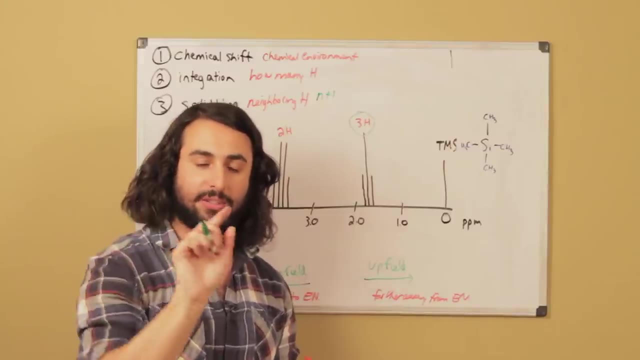 and so basically what we are saying is: let's say we have a hydrogen that is generating some resonance. it's generating some resonance, but then if there is a neighboring proton that acts like a little magnet. so let's say we are looking at a proton of one carbon over. 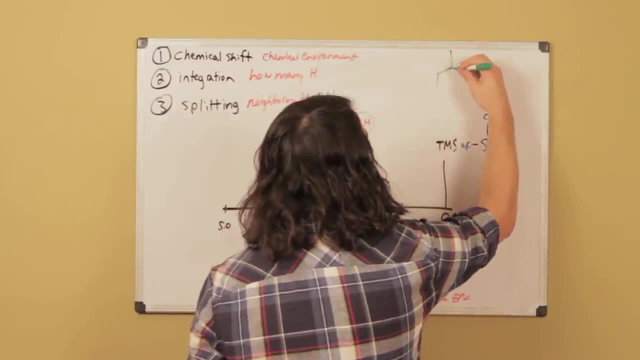 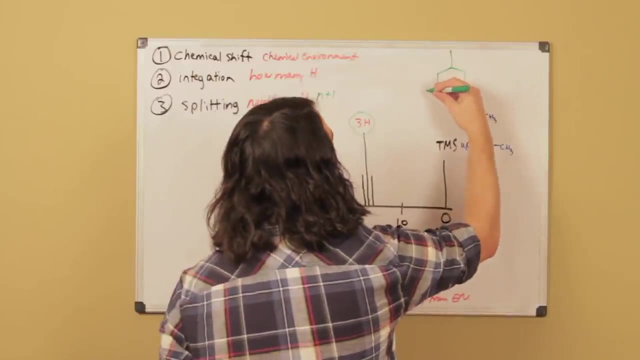 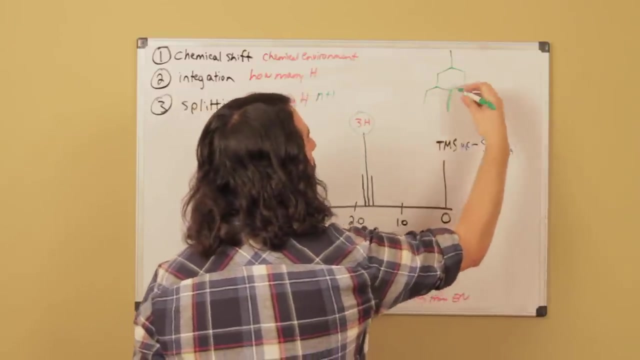 and that proton will split this one into two resonances. now let's say that there is another. there is a second neighboring proton that will split this into two resonances and this into two resonances. so we will have an overlap there and that one will be more intense. 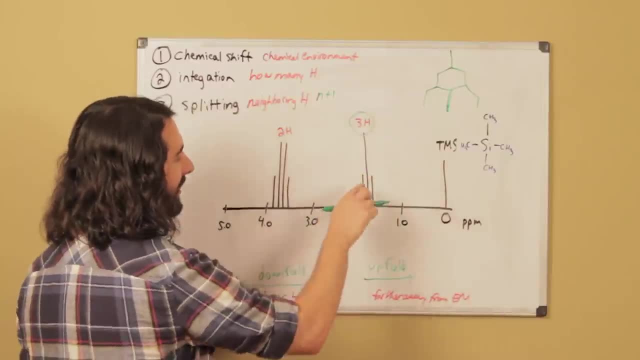 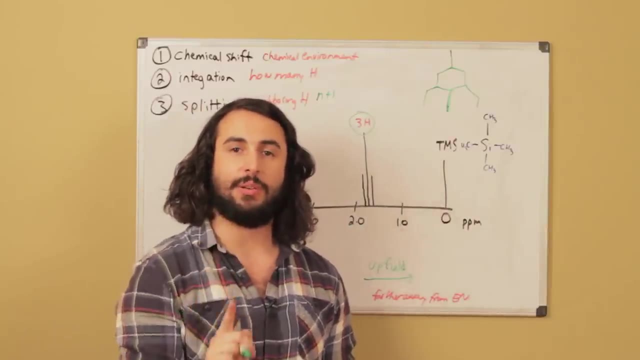 this middle one will be more intense, and so that's why we see something like this we have: the middle one is the longest, but, at any rate, we are seeing that an individual resonance that is generated by one proton will be split into smaller, a series of smaller peaks. 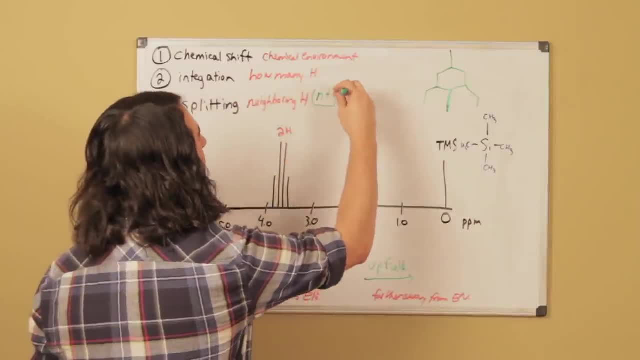 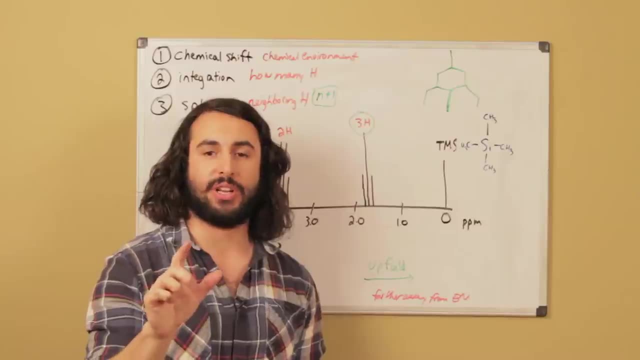 by neighboring protons, and so specifically, it will be split into N plus one peaks, where N is the number of neighboring protons. so if we have some chemically equivalent protons with, let's say, two protons next door, it will be split into three peaks. 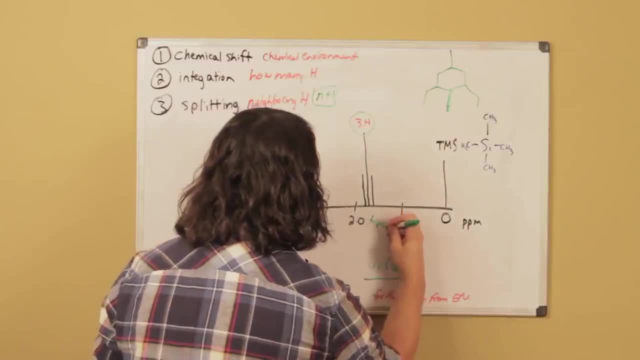 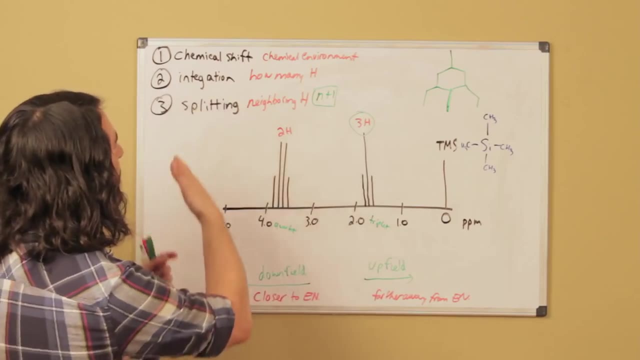 or a triplet. so this is called a triplet, this would be called a quartet. we could have a singlet, we could have a doublet. so that's splitting. that is telling us the number of neighboring protons. so that's the three. those are the three bit of data. 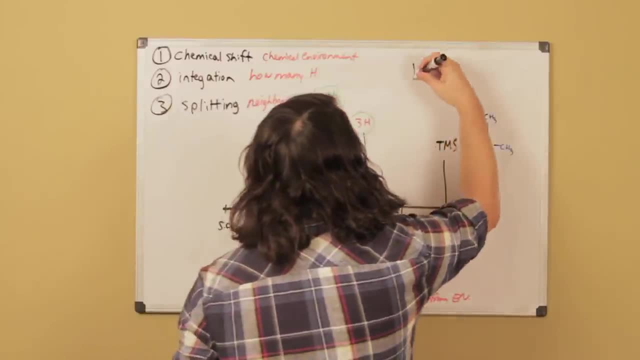 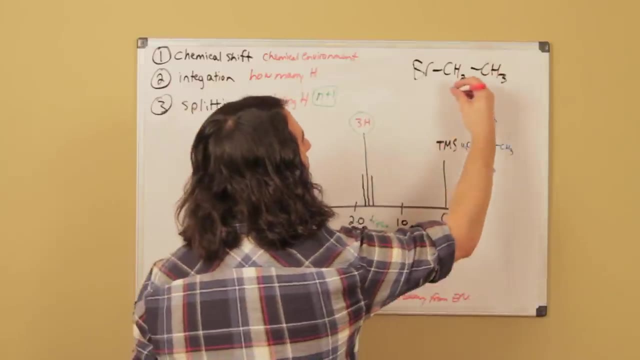 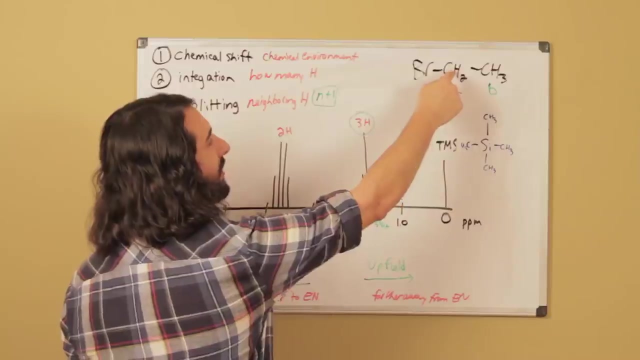 so now let's look at the structure of what this actually is. what this actually is is bromoethane and let's assign the peaks. so what we need to understand is that we have two different. we have two different resonances to expect, because these two protons are chemically equivalent. 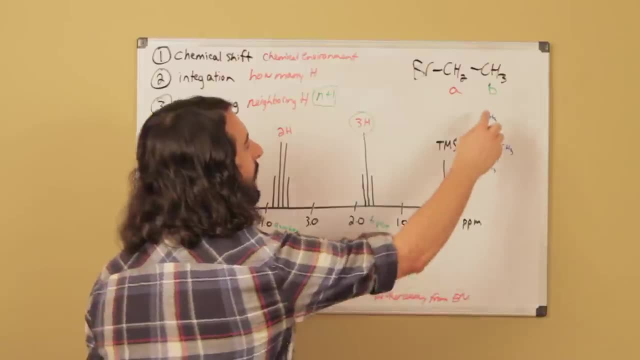 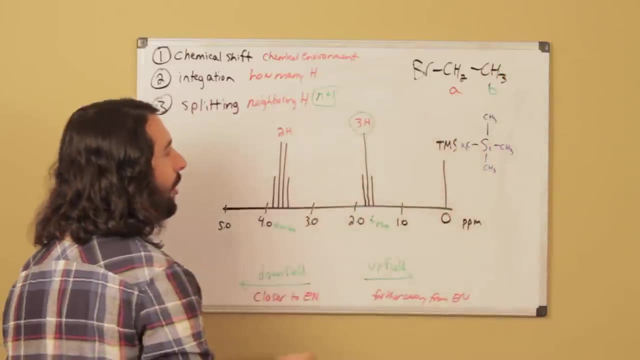 usually the protons on the same carbon are chemically equivalent, and then we have three that are chemically equivalent over here, so let's look at this one first. we're saying that these are three of them, so we better have it integrated to three. so it's probably going to be this peak. 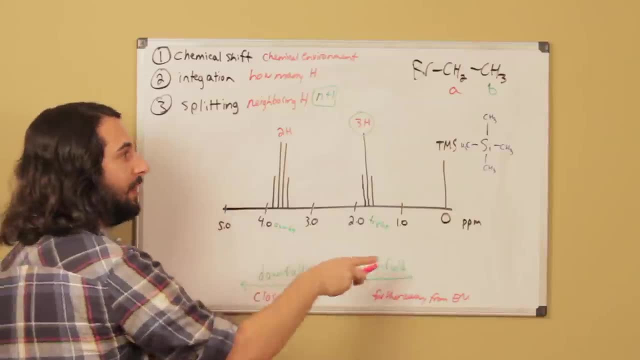 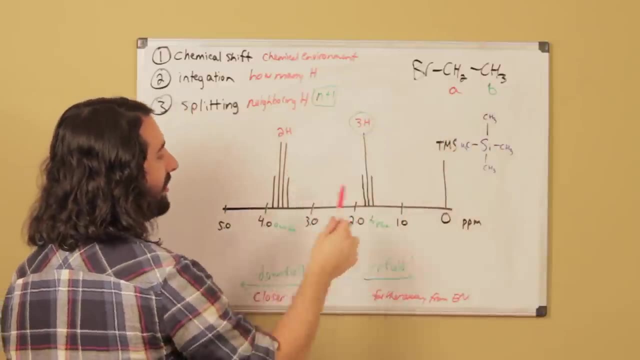 in addition, it's further away from the bromine, so it should be more upfield, and then it's going to be split by the two neighboring protons into a triplet, because two plus one is a triplet, so we have a triplet that is integrated to three. 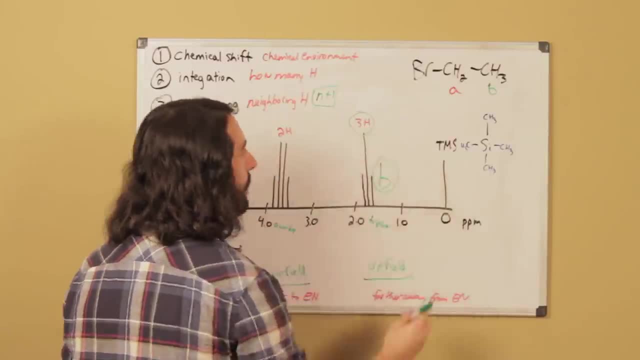 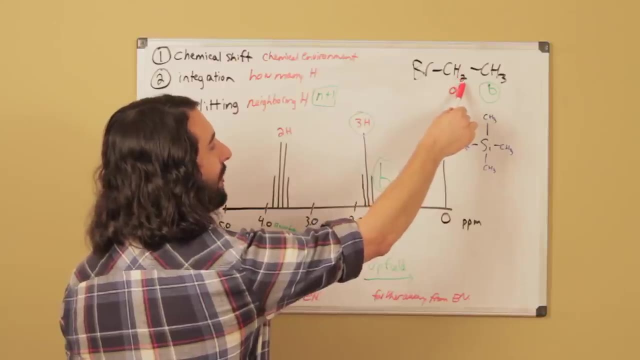 that is more upfield. so this peak certainly corresponds to B. then, looking at A, we're saying that we need to look for a peak. that number one is integrated to two because there are two protons. also it should be further upfield because it's closer to the bromine atom. 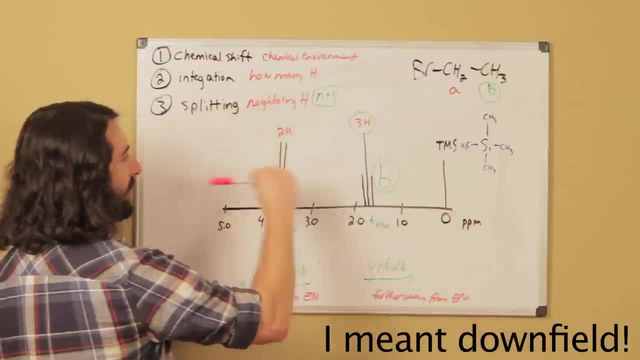 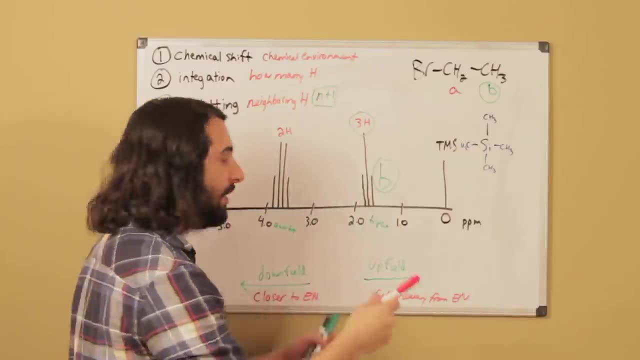 the bromine atom is going to deshield those protons, so that's further upfield, and then additionally the three neighboring protons. three plus one is four. it should be split into a quartet by those neighboring protons. so this certainly is going to be A. 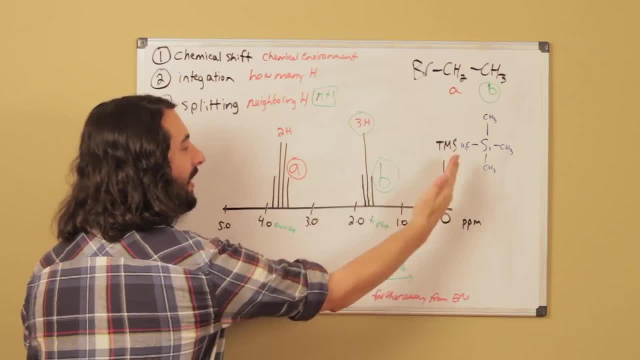 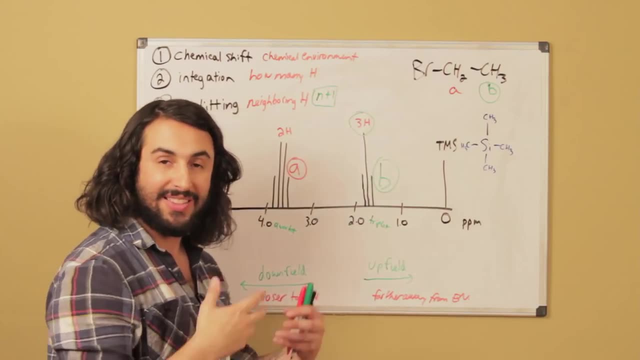 so, just to reiterate, we have chemical shift. where is it sitting on the spectrum? we have integration- how tall is it more or less? which refers to the number of protons that are generating that resonance, and then the splitting pattern, which tells us how many neighboring protons there are. 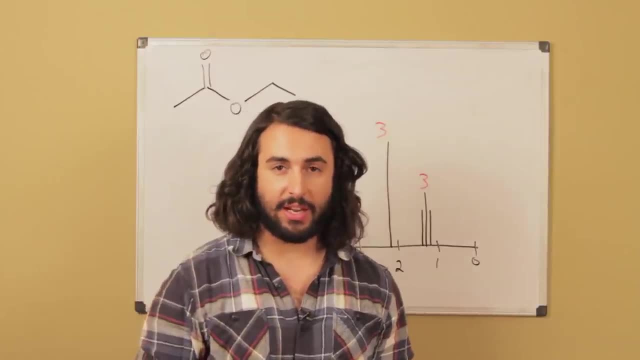 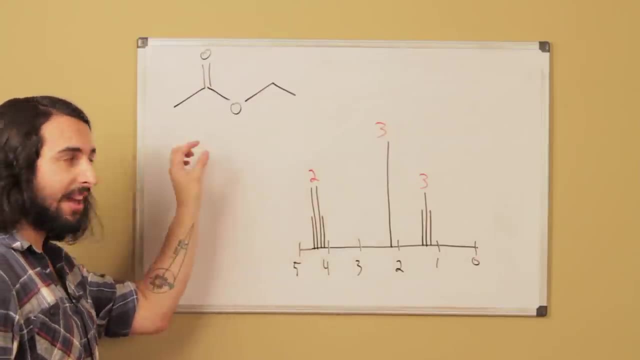 ok, let's look at one more sample spectrum to make sure that we can assign these NMR spectra. so let's say we're looking at this compound and we want to match the match the protons to the peaks that they correspond to. this is probably going to be something you'll do. 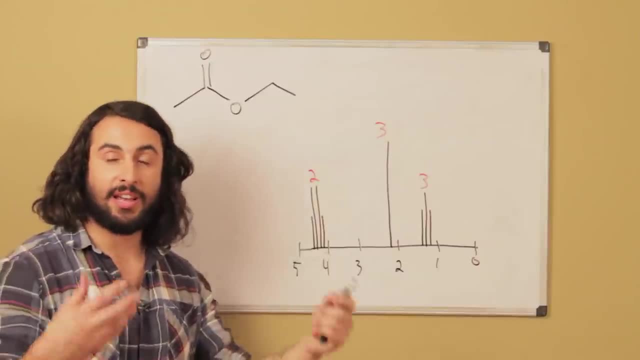 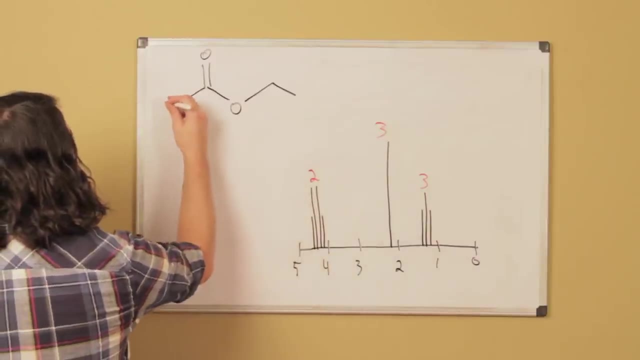 in any organic chemistry course you'll be given a compound and a spectrum and the problem will say: match the protons to the peaks they correspond to. so first of all let's make sure we understand where the protons are. so we've got three there. we've got two there. 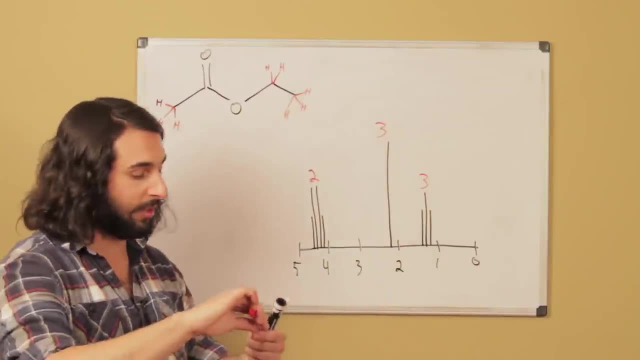 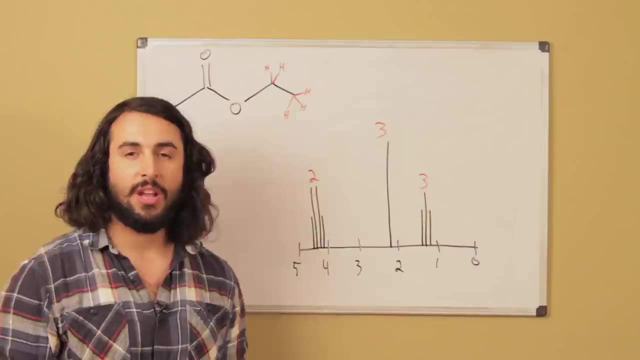 and we've got three there. we definitely have to be able to do that, otherwise this is going to be extremely difficult. now we know that for the most part, at least at this early stage of analyzing NMR spectra, let's just say that all the protons 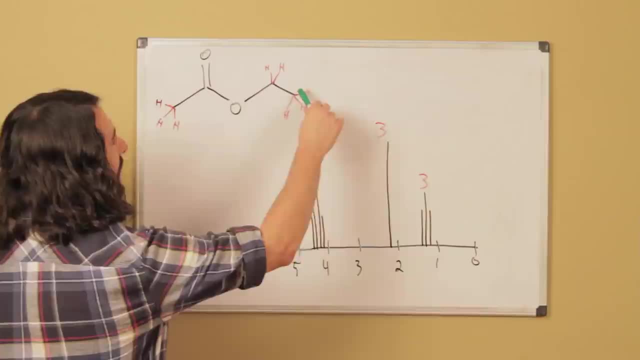 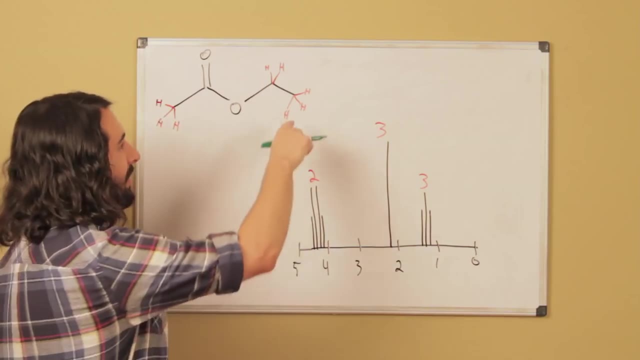 on an individual carbon are going to be chemically equivalent because, let's say, we've got these three protons on this methyl. as this bond is rotating, there's no spatial differentiation, it doesn't matter if one's down or up or whatever, as they spin around like a top. 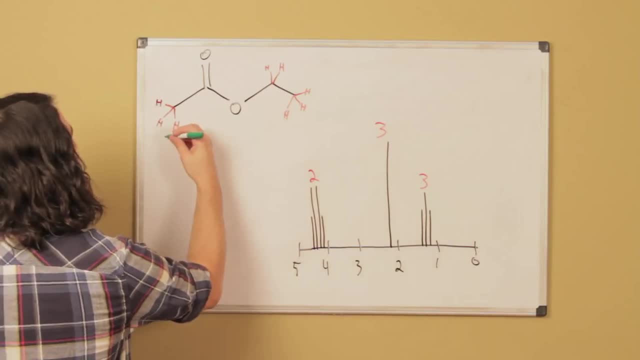 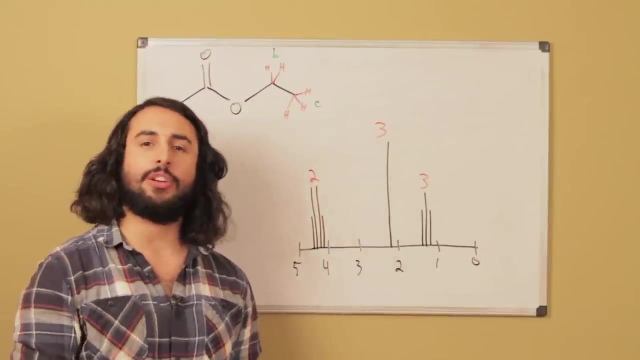 they're all seeing the same chemical environment. so these are all the same. what's called them A? these two are the same. what's called them B? these three are the same. what's called them C? now, there's one very good method either. we could just try to assign straight off the bat. 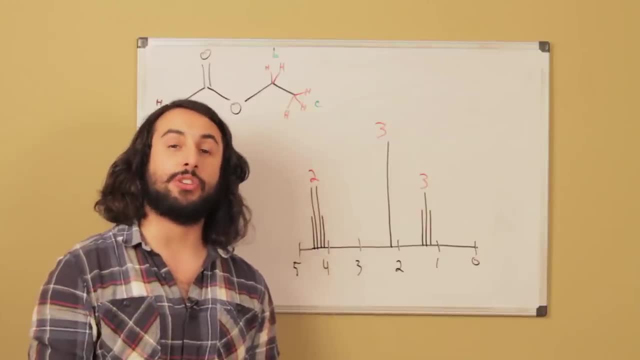 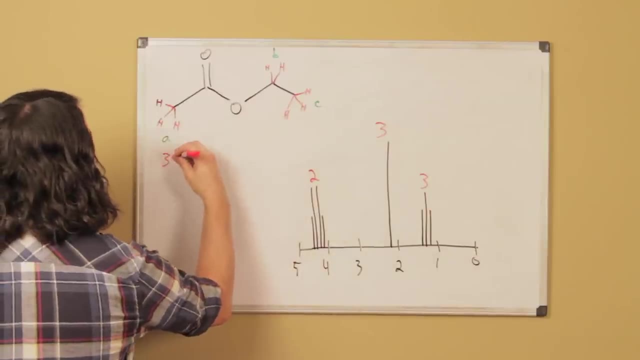 but first, just to be a little more thorough, let's make predictions about what we could expect from each resonance. so, looking at A first, we know that this is going to be integrated to three. we know it's going to be integrated to three because there are three protons. 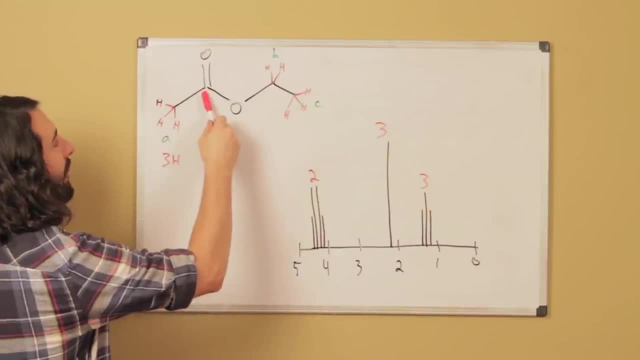 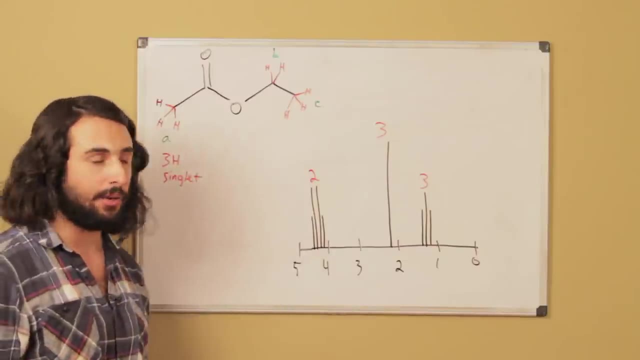 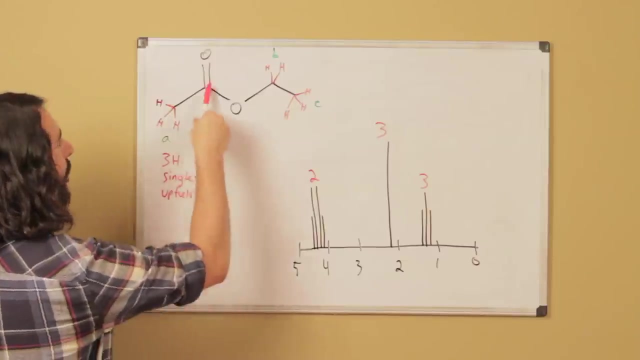 then let's talk about splitting. there are no neighboring hydrogens, so it will not be split at all. we are expecting a singlet here. and then, lastly, we expect it to be relatively upfield, because it is near a carbonyl carbon. now, if we want to be very specific with our predictions, 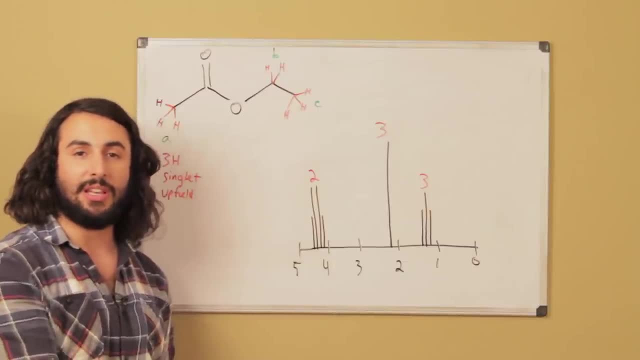 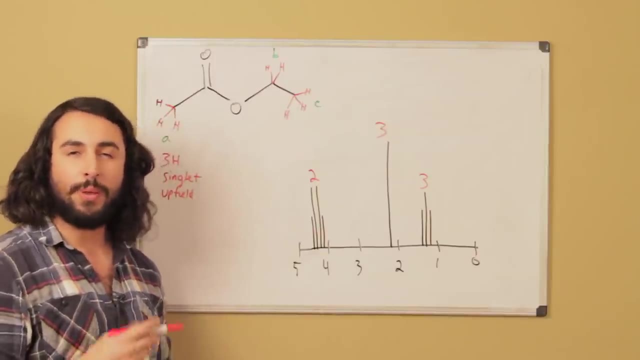 we could consult a table that would tell us the exact ppm to expect for hydrogens next to a given functional group, or whatever it is. so we may not even really need to, though, because we have plenty of information here. this is a very simple molecule: there's only three peaks. 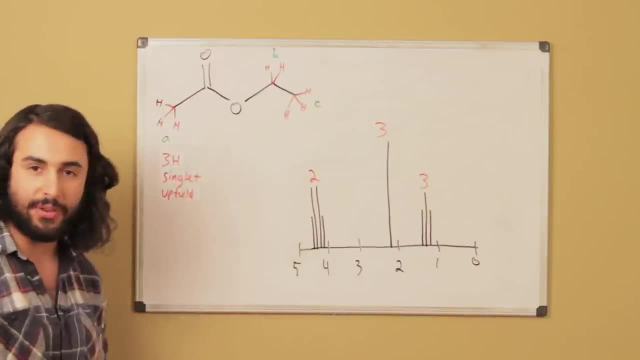 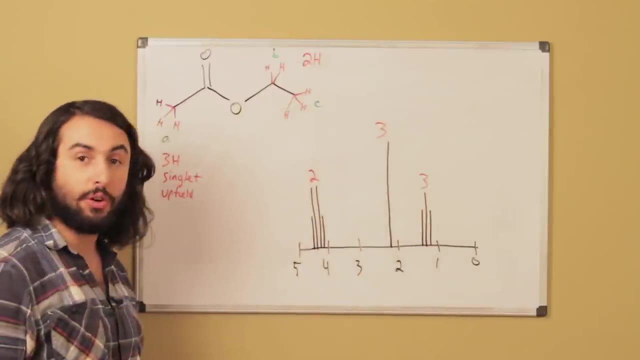 so this is going to be enough. a 3H singlet that is relative to a 3H singlet relatively upfield. that's plenty of information. then over here. we know that there's two hydrogens, so we expect that that resonance is going to be integrated to two. 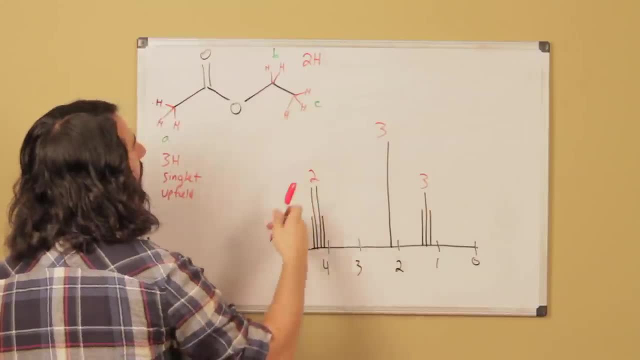 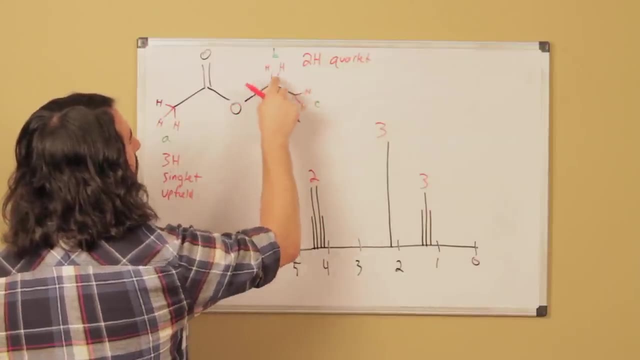 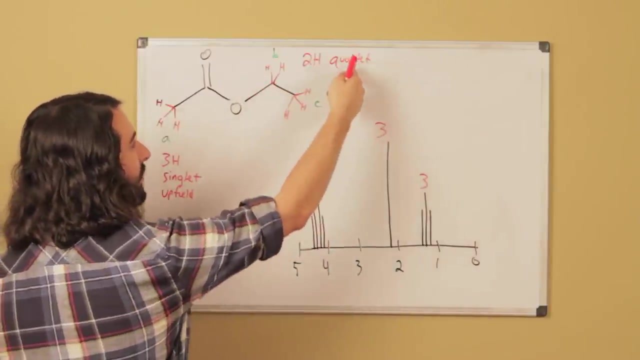 because there are two of them, and then we expect it to be split into a quartet because there are three neighboring hydrogens. so here's the hydrogens we're talking about. the neighboring ones are right here. there's three of them, and so 3 plus 1 gives us 4, a quartet. 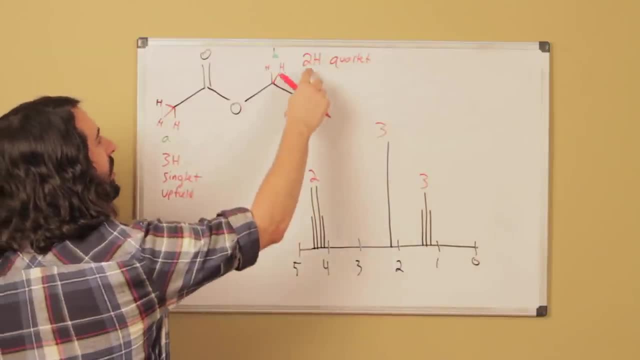 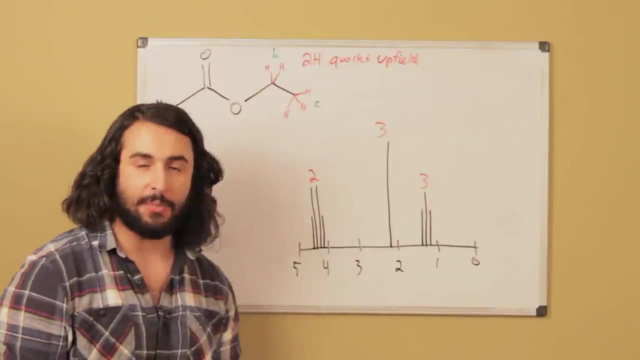 there are no hydrogens over here, that's an oxygen, so a 2H quartet. that should be again relatively upfield because these are adjacent to an oxygen atom. an oxygen atom is very electronegative. it has a lot of electron withdrawing capability, so those should be relatively deshielded. 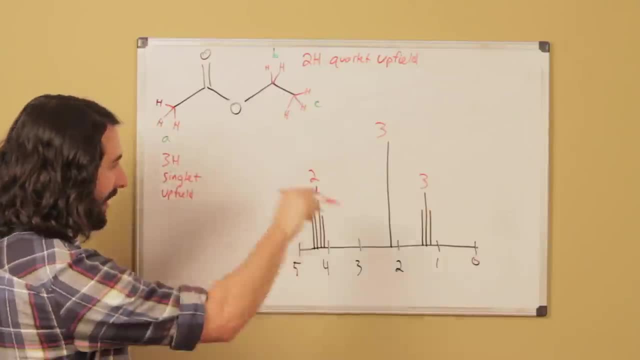 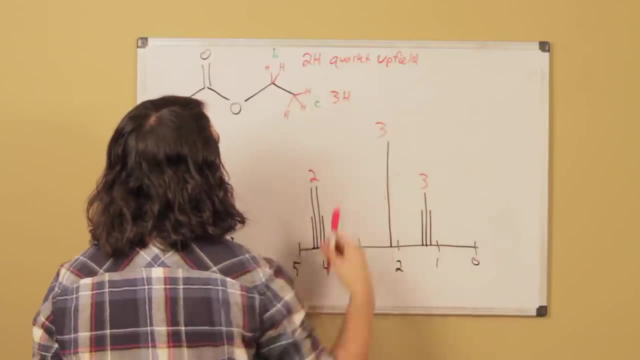 and relatively upfield protons, or the resonance that corresponds to those protons. then, lastly, right here we've got three chemically equivalent protons, so we should expect a peak integrated to three. we should expect that it is split into a triplet because we have two neighboring hydrogens. 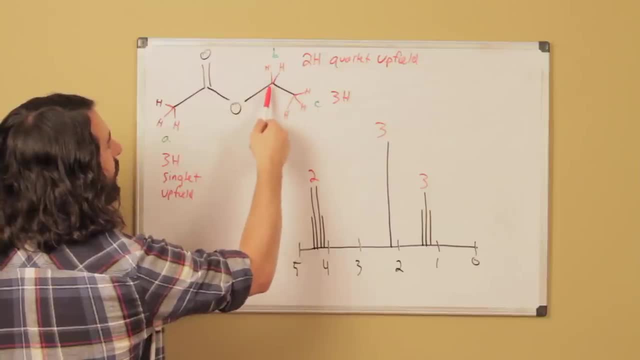 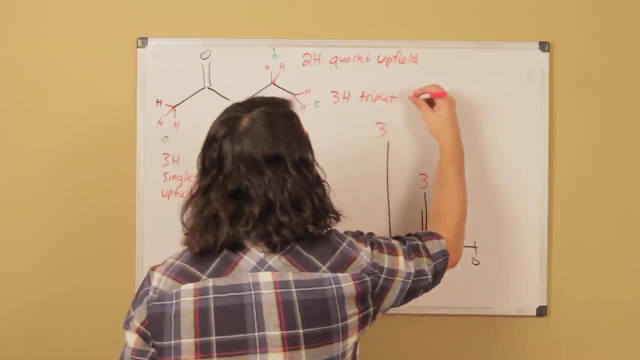 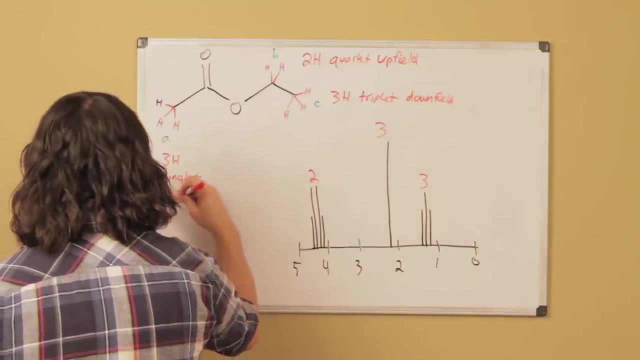 so n is 2, n plus 1 is 3, so this resonance should be split into three smaller peaks, or a triplet, and then we should expect that it is relatively. oh, you know what? I think I mixed up. what I meant was downfield. 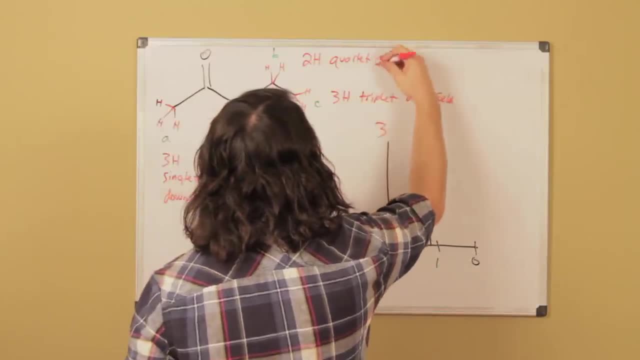 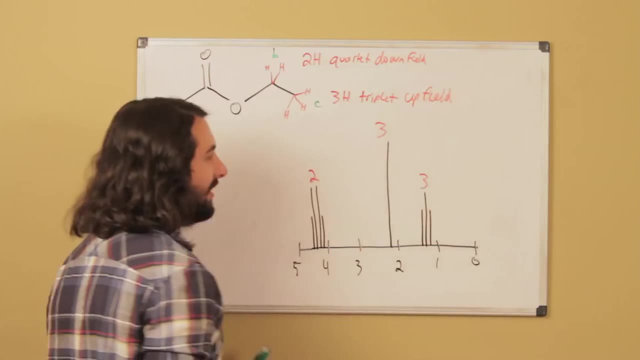 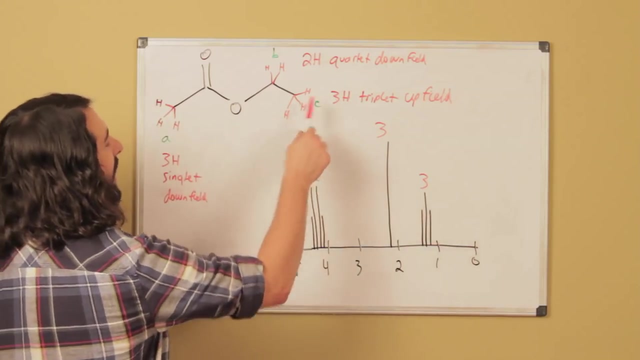 here and upfield. this should be relatively upfield because it is not near an oxygen atom or any electron withdrawing group, so it is relatively shielded. it will stay relatively upfield. so we have a 3H triplet upfield, so now this is going to be very easy to assign. 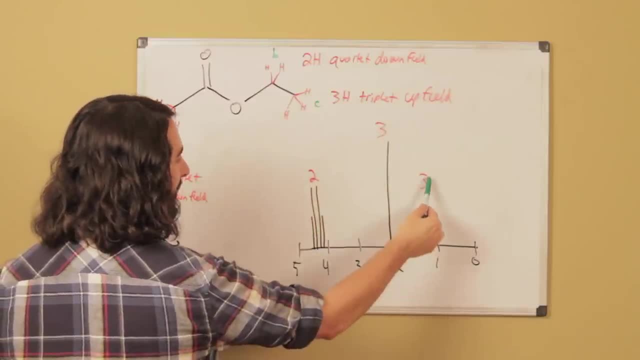 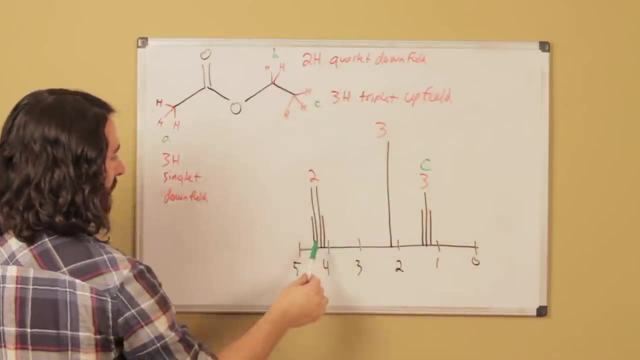 so let's say, here we have a 3H triplet upfield. well, this is integrated to three. it is a triplet and it is upfield, so this is certainly resonance C. here we have a 2H quartet downfield, so here it's integrated to two. 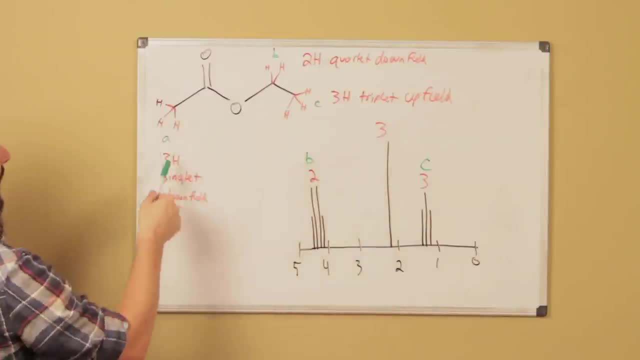 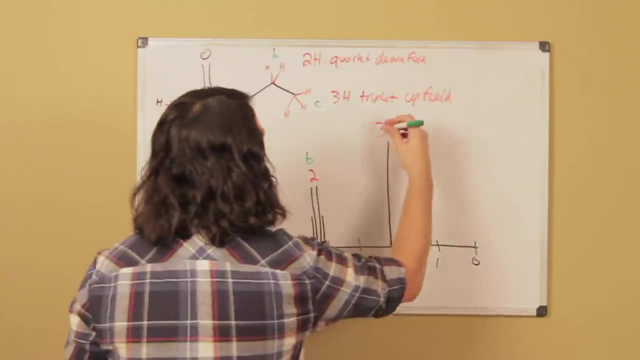 it's a quartet, it's downfield, that's got to be B, and then we have A. we have a 3H singlet may or may not be downfield, it's right there in the middle, and so that is certainly going to be peak A. 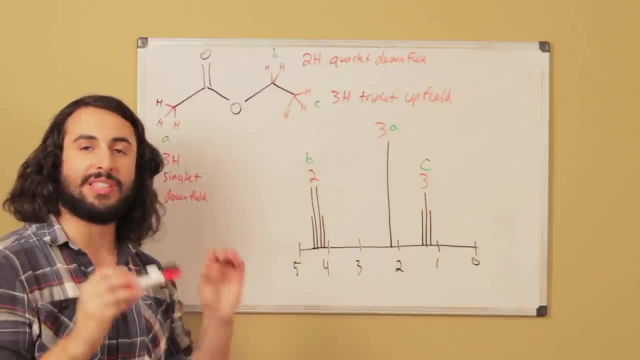 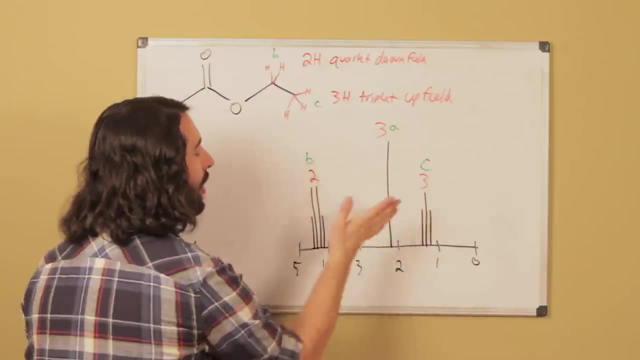 so, once again, when we are looking at a molecule and we are trying to assign resonances to the protons that they correspond to, we are going to be looking at three things. we are looking at chemical shift, we are looking at integration and we are looking at splitting. 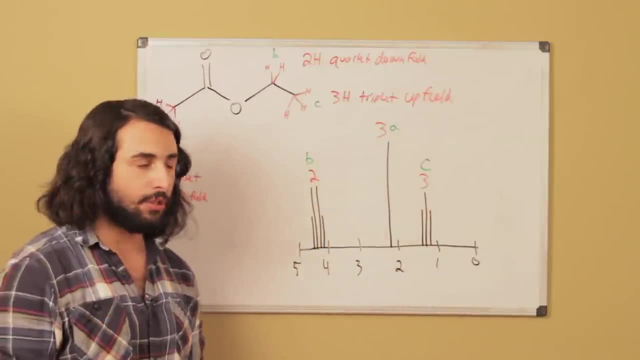 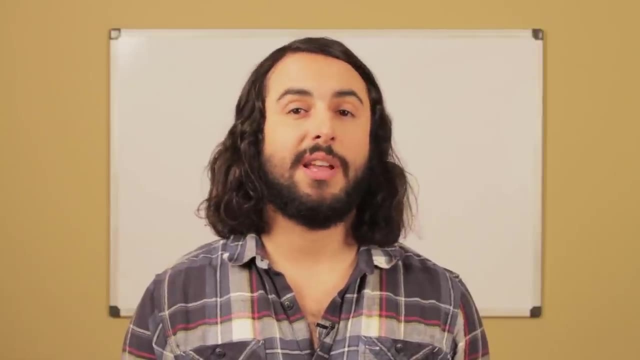 and all we need to do is get enough data to be able to assign those peaks accordingly. thanks for watching guys. subscribe to my channel for more tutorials and, as always, feel free to email me.